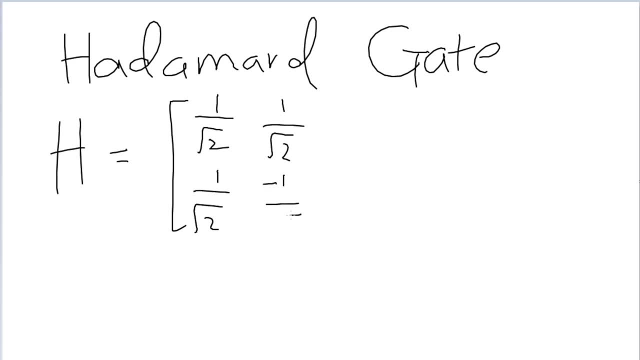 1 over root 2, and our lovely negative 1 over root 2 wildcard in there. Now, of course, this is quite a lot to write, And actually we can simplify it down just to be 1 over root 2. 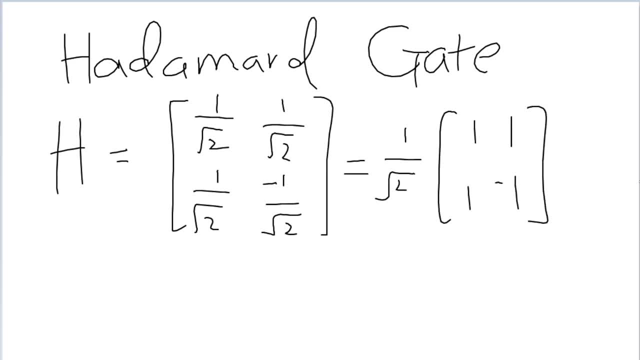 multiplied by a matrix full of positive 1s and a single negative 1 for our wildcard, That is, our Hadamard gate. Now the question is: what does it actually do to the qubit that we're applying it to? In order to truly understand what occurs, let's actually consider this in a case-by-case. 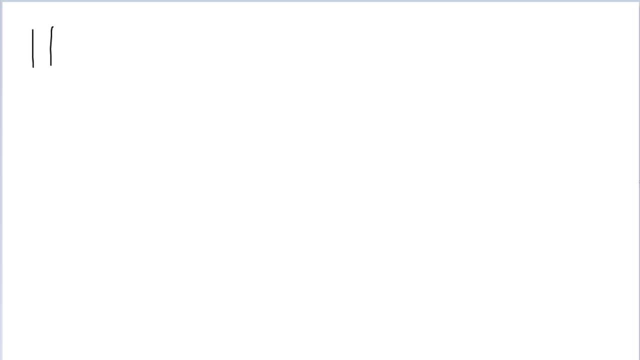 scenario. So let's begin by applying our Hadamard gate to our 0 vector. Now recall: 0 here is going to be represented as oops, that should be a positive 1.. Right, this is our Hadamard gate. It's going to be represented as 1: 0 vector of 1: 0.. And so we 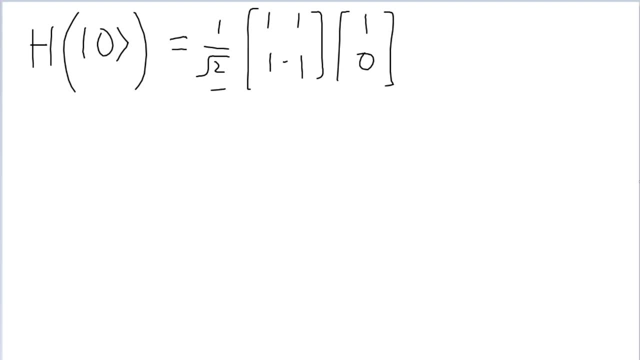 see, here we have a case, actually a combined case, of scalar multiplication with matrix multiplication. So let's do matrix multiplication first Scalar multiplication, basically just kind of a distribution problem. So what we have here, if we write out what is occurring, we have 1 over. 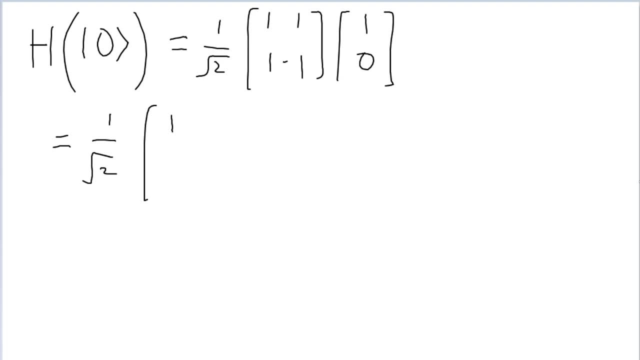 root 2 multiplied by 1 times 1, plus 1 times 0, which is 0. And then we have 1 times 1,, 1 times 1, right, which is 1 again, plus negative 1 multiplied by 0, which is 0. So we have 1 on the bottom, as 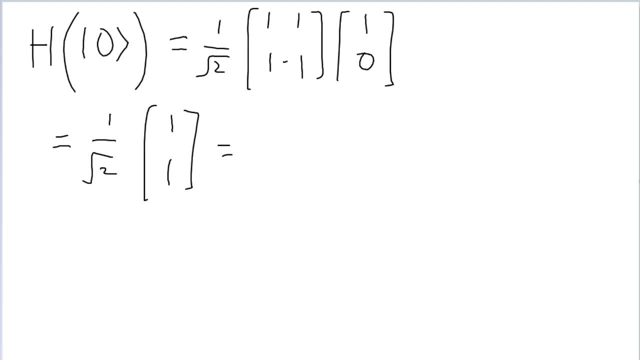 well, And so this is the result. And you might be saying, all right, that's wonderful, What can we get from this? We have 1 over root 2. And actually, if we rewrite this out, you will see that this is: 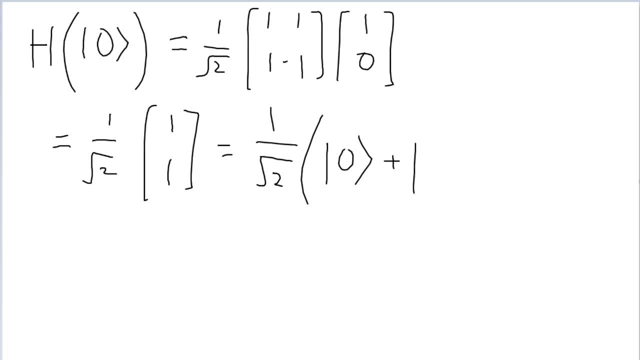 equivalent to 1 over root 2, being multiplied by our vectors representing 0 and 1.. Which is interesting, because we started out with this lovely little friend right here, And what we've resulted in, what we have got in return, is fundamentally a qubit that is existing in. 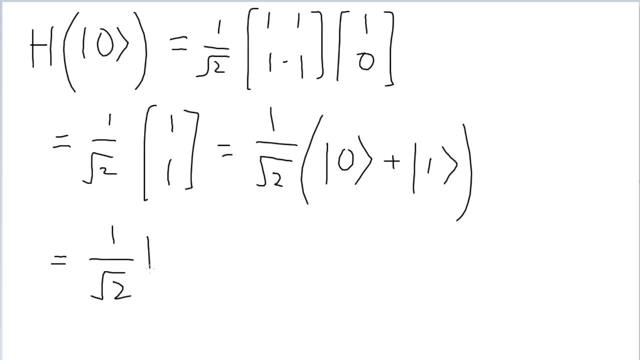 superposition, Because we see here that, rather than knowing for sure and with definite confidence that our qubit is pointing in direction 0 or has value 0 in this case, we now can only say that our qubit has a 1 half probability of being measured to be come out to be equal to value 0. 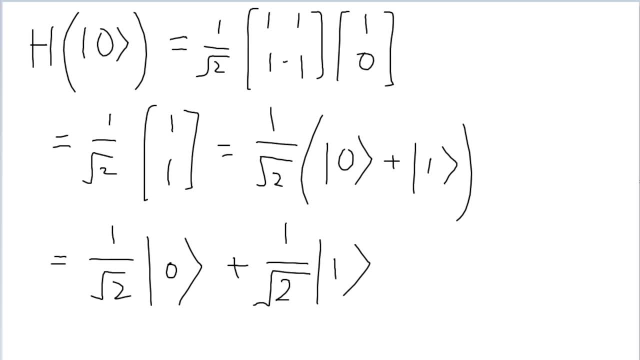 in a way that is not. So. we have 1 over root 2 multiplied by 1 times 1, which is 1 over root 2 multiplied by 1, half probability of being measured and coming out to be value 1.. Again, this relates: 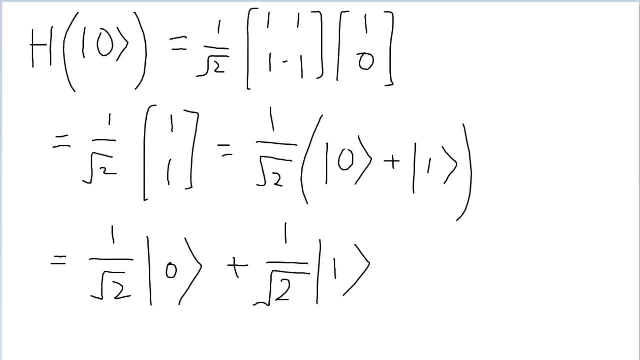 to the probability of the twos, And so clearly we've taken this initial qubit right here and put it in superposition. So what happens if we, and what occurs if we attempt to apply this Hadamard gate to our vector or a qubit that has been measured to be in direction 1? Well, quite simply. 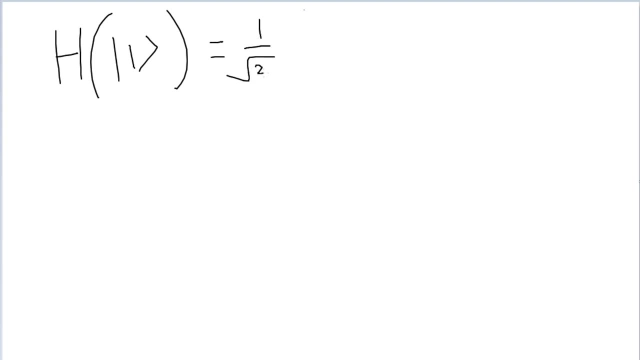 if we rewrite out all that we have had in the past, we have our Hadamard gate walking through the same exact steps of applying it to this qubit here. In this case, this qubit is denoted as 0, 1, right. 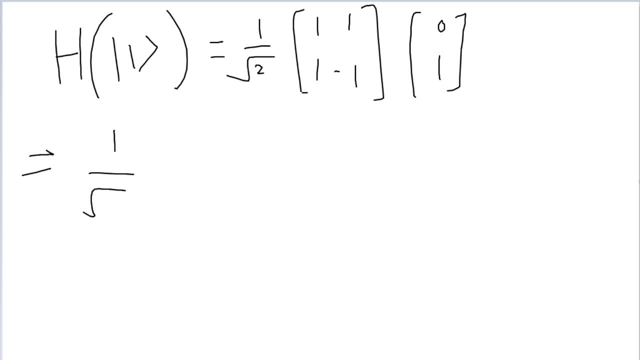 We see, rather than being 1 over root, 2 multiplied by 1, 1, we actually see that is 1 and I do believe negative 1 down here, which gives us 1 over root 2 being multiplied by our vector. And let me write. 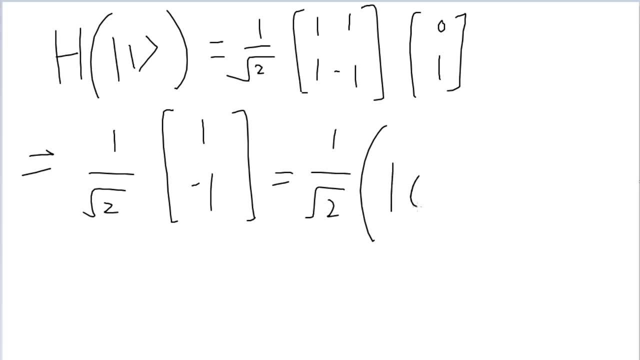 this a little bit neater, Being multiplied by our vectors 0 minus 1.. And now you might say, all right, so you know what's the big difference. So your big deal, you know, squaring probability amplitudes regardless of whether it's positive. 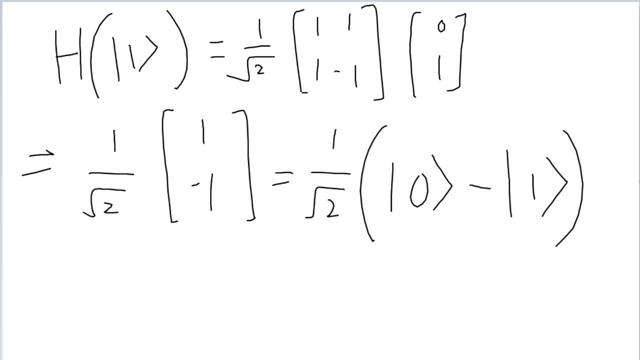 or negative, will still give us the same exact answer. And the answer is: well, this kind of goes back to our idea of equivalent state factors, and whether or not you're just nicking only one of, perhaps like two terms within our linear combination will actually do anything. And yes, 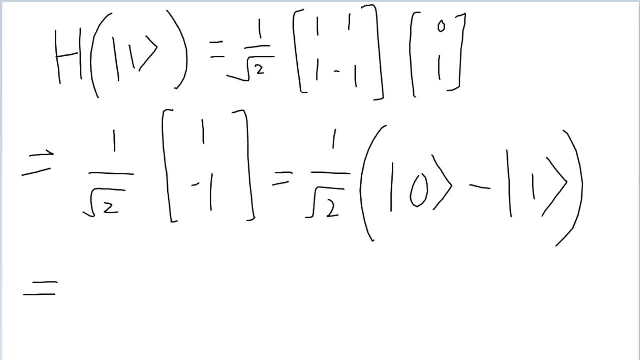 it does, It changes the technical direction in which we're looking at it. And so if we say, all right, so what does this linear, new linear combination look like? We see again that it has a one-half chance of being measured to be in direction 0 or a vector. And so if we say: 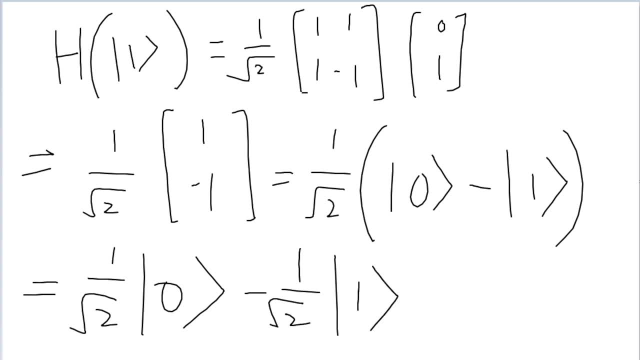 oh, it's going to be a value 0, one-half chance of being a value 1.. And, as a result, we've taken this qubit and put it into a superposition, And that is actually largely what this Hadamard gate. 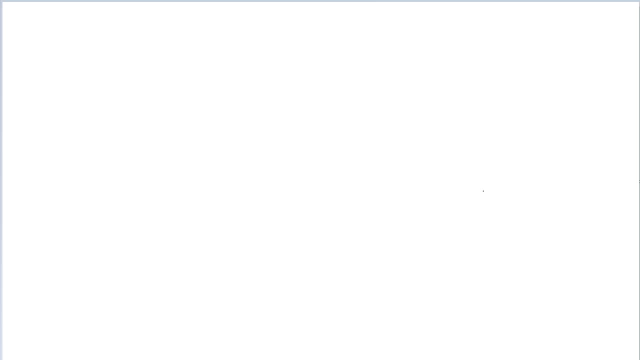 is used to do. It takes our qubit and it puts a qubit that we know, you know that we have a definite value of, and it puts it into a superposition of some sort. So if you are to ever encounter in, perhaps like a quantum circuit of some sort, perhaps you'll see it denoted as like: 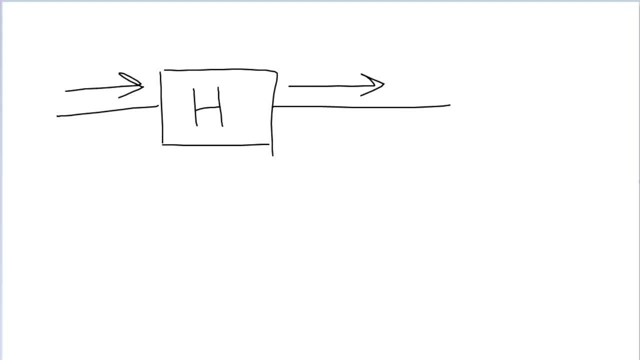 a line, right? This is our input here, This is our output. a single line here in this case, because it is again possibly a one qubit operation, technically speaking, right, And so you see a bit of a box with an H on it. So if you ever see that we have a Hadamard gate on our